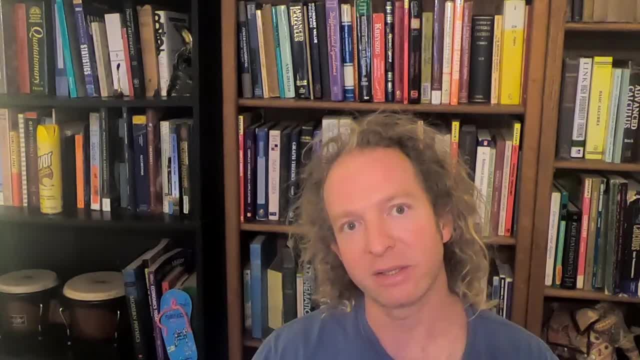 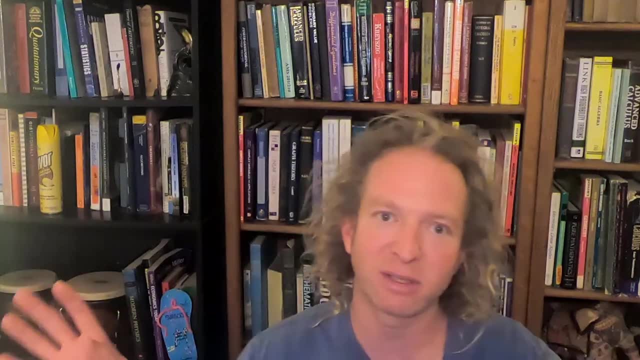 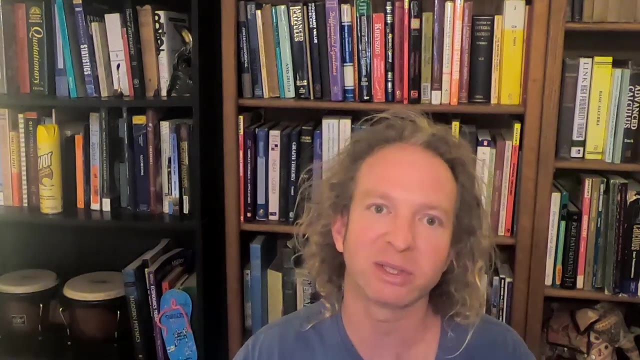 In this video I want to talk about something that is a little bit different, and people talk about this and they say: you see it all the time, it's something that's kind of popular, and they say that math helps with what they call analytical thinking, problem-solving skills. 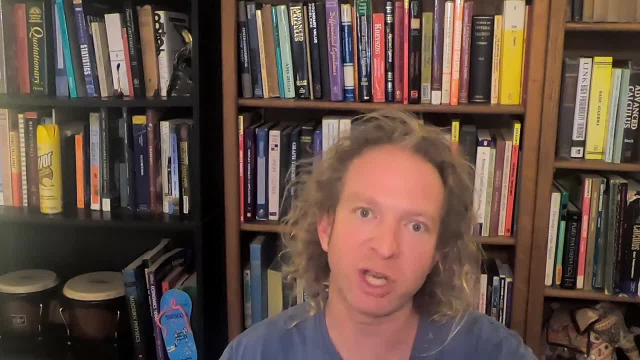 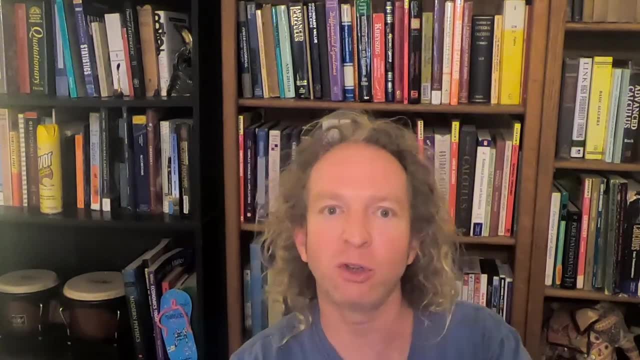 And so when people say that, I think a lot of times people immediately jump to: oh yeah, if you're good at math, when you get a job somewhere working for a company, you'll be good, you'll be a good problem solver, you'll be able to figure things out. Sure, that's true, but that's. 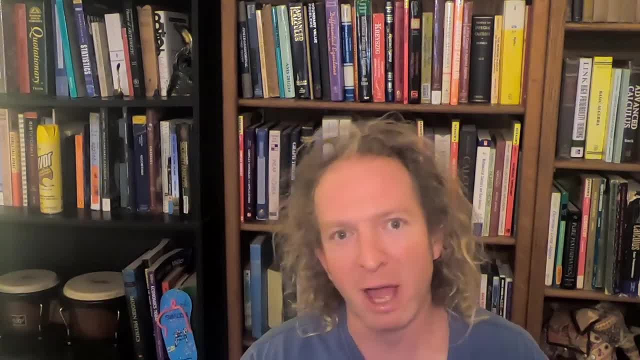 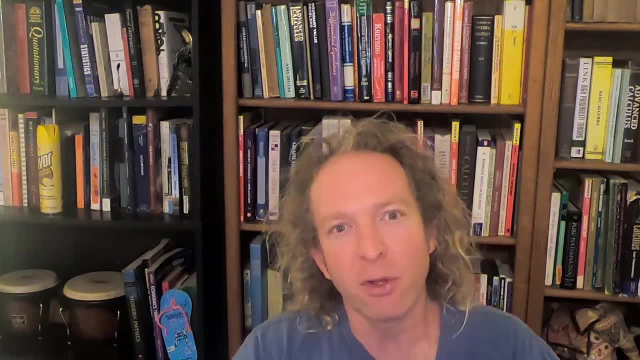 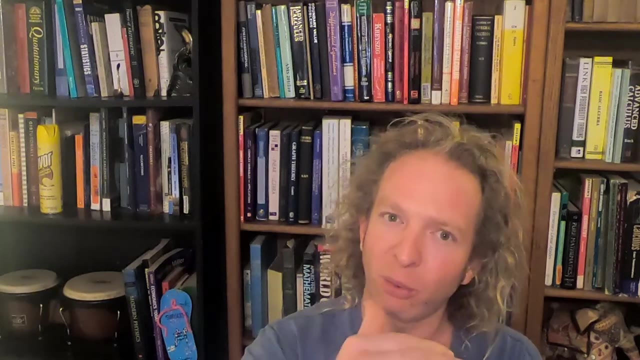 not what this video is about. This video is about how math can actually help you with your personal life problems. right, Math is a huge problem-solving process. right, We have to actually read the problem, understand the question, and then we have to have some background knowledge. 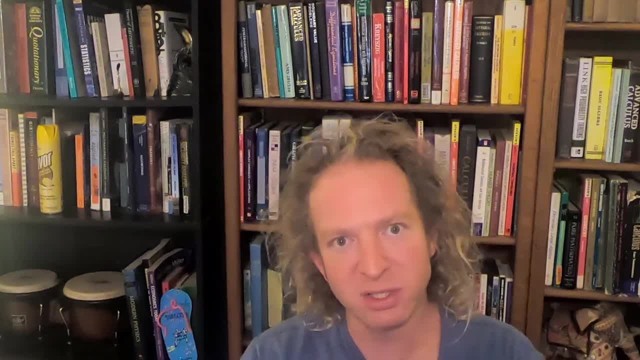 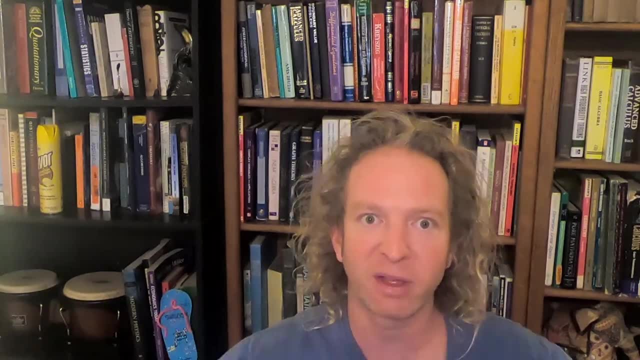 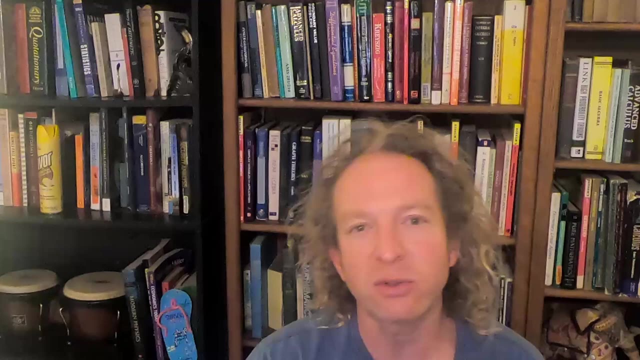 on that math, math problem. And then we have to use that knowledge to somehow correctly from that knowledge deduce certain steps and come up with a proof, right? So the same is true in mathematics and in life problems, right? If you're talking to a person and there's a conflict, if you have a. 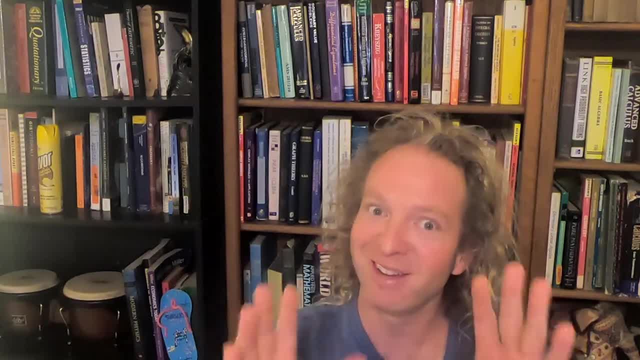 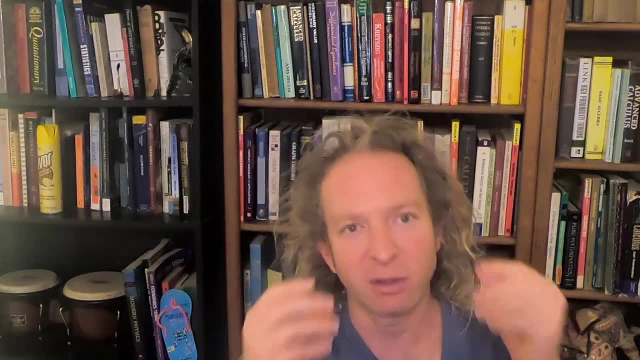 problem with a person. right, Assuming the person is logical. right, It's the same thing. right? You're talking to the person you know, you listen to what they're saying, you listen to their words and you have some background knowledge with this person. 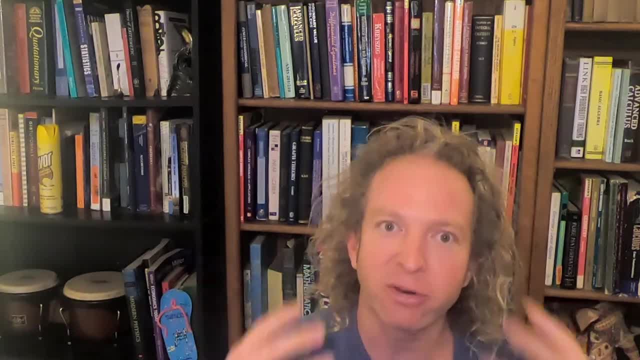 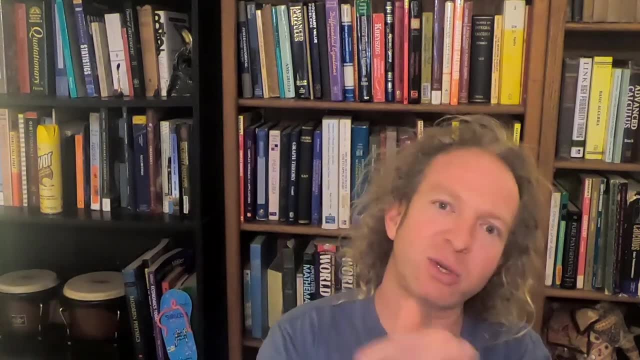 right, And so from that you can gather your thoughts and then from there maybe come up with a viable solution to whatever the problem is. So I just used a person, another human being, as an example. But if your car breaks down, or if you need to buy a new car, or if you're thinking, 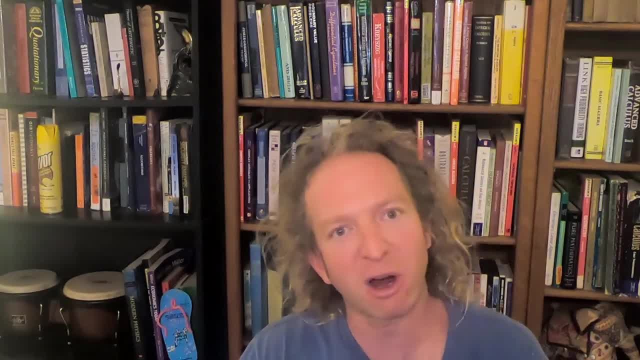 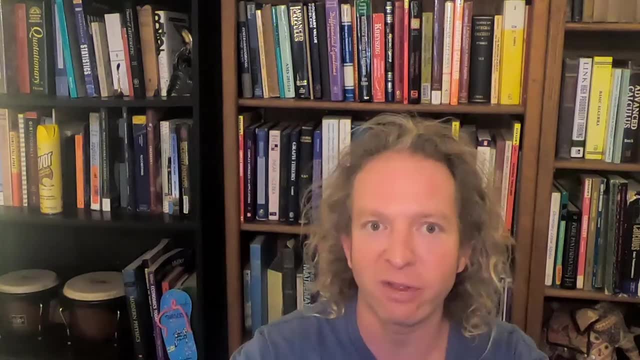 about buying a house, or if you're thinking, hmm, should I get better car insurance? right. Regular life decisions- Oh, should I rent an apartment here or should I rent it over there? Things that we all have to make. decisions on Where to open a bank account- right. 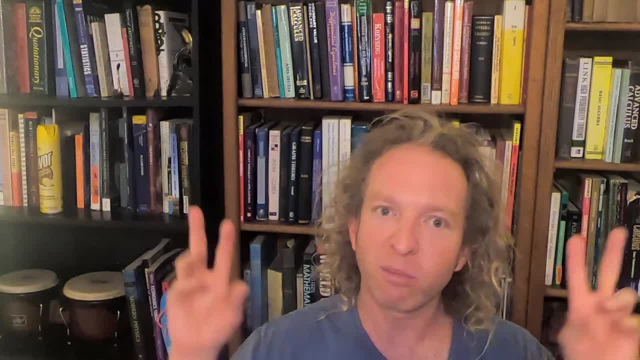 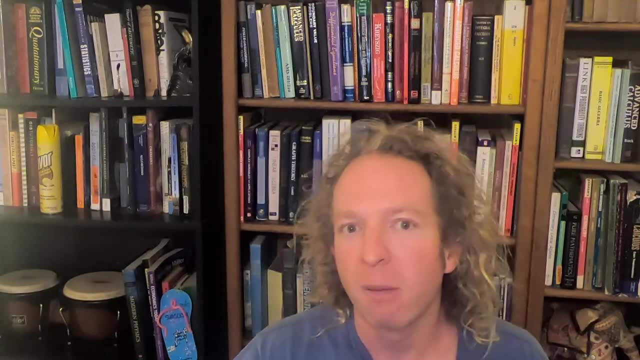 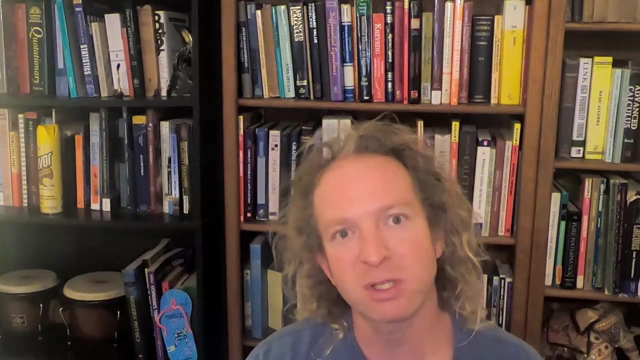 All of these things, these are life decisions, these are life problems, quote-unquote- and our mathematical studies help us solve those problems. Before I started college, I was completely different in my thinking and when I was done with my math degree, even with just my undergraduate- 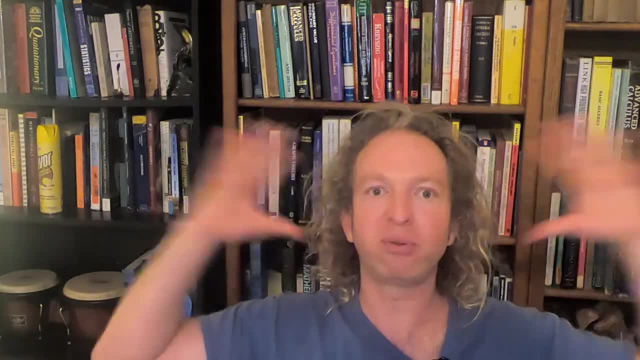 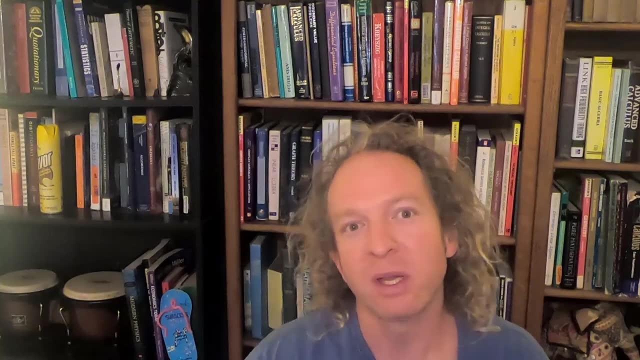 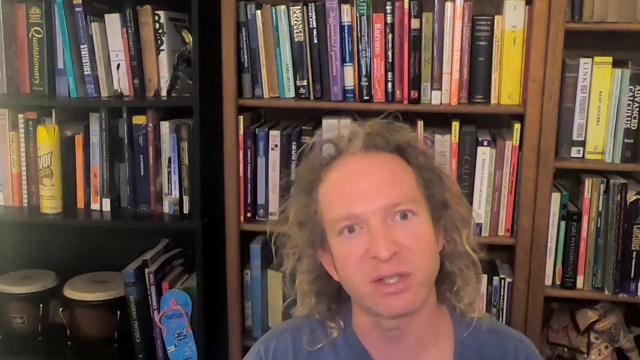 degree. the way my mind worked was completely transformed. The way I talked was completely transformed. Math totally changes the way we think and it totally helps us with life problems and with everyday decisions, right? So if you're watching this video and you're thinking, 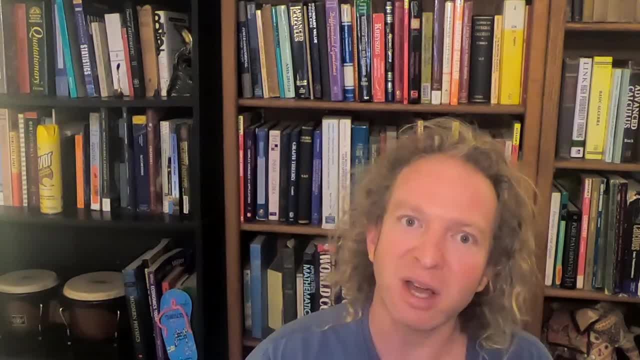 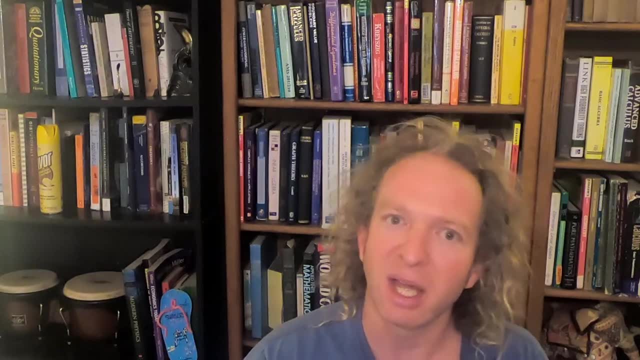 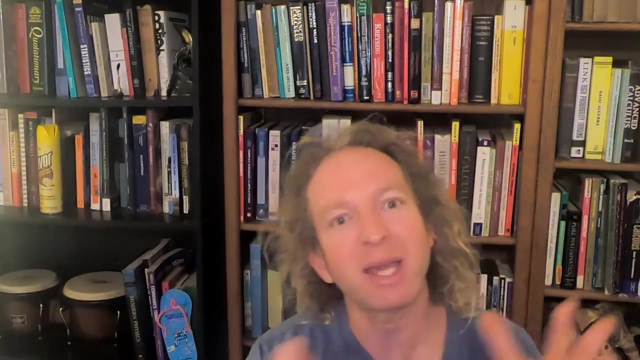 yeah, maybe it does, You're right. You're right, It actually does. So think about that Next time you have to make a decision in your life. think about it carefully and just think logically, And from that you should be able to use what you've learned in math and somehow apply it. 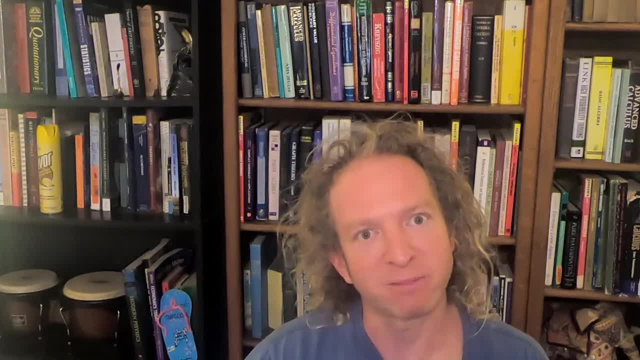 to your life. So until next time, take care. 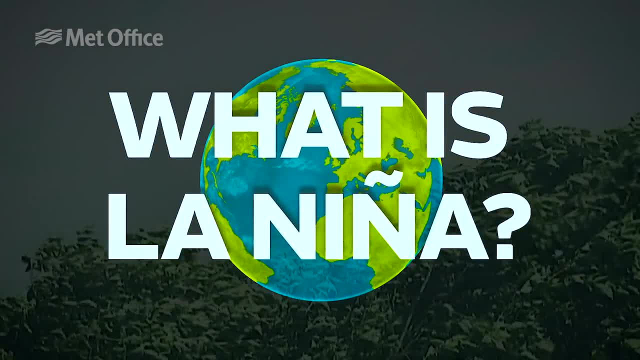 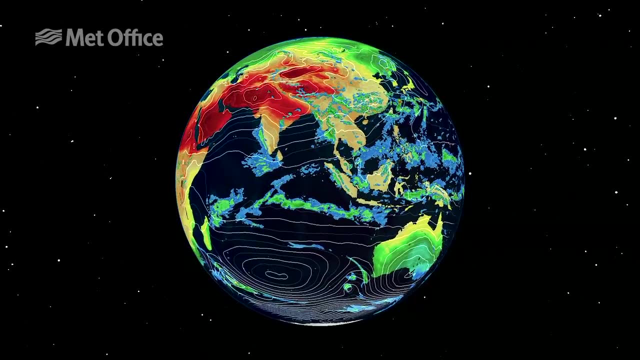 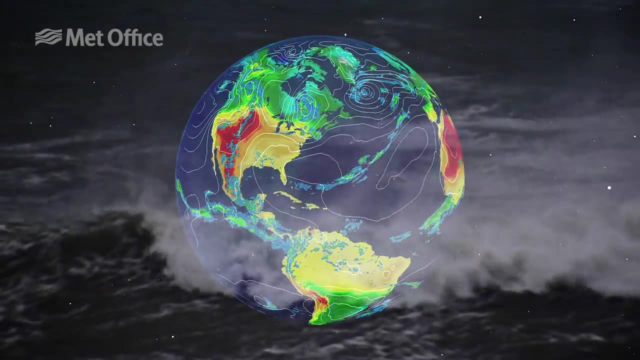 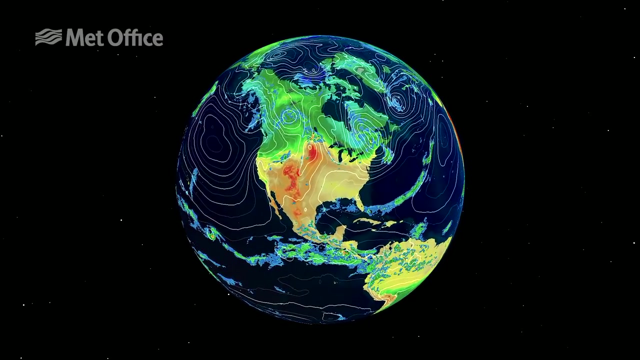 El Niño and La Niña are terms for climatic events originating in the tropical Pacific as part of a naturally occurring cycle. Such events are a consequence of strong interactions between the ocean and the atmosphere. The cycle transitions between a warm El Niño and a cold La Niña phase. Both La Niña and El Niño tend to peak during the northern 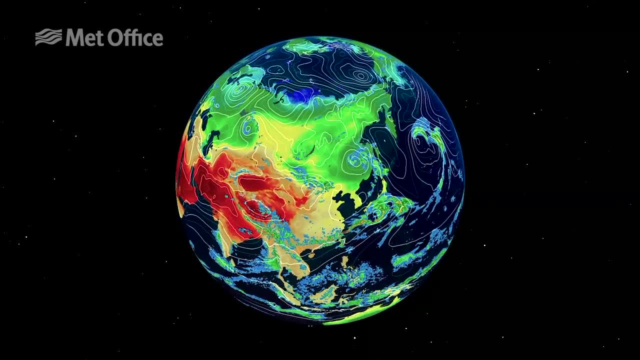 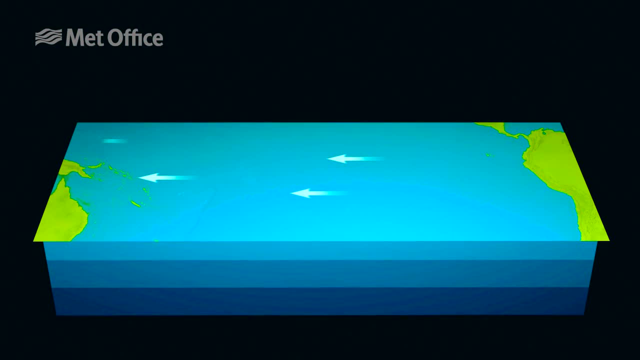 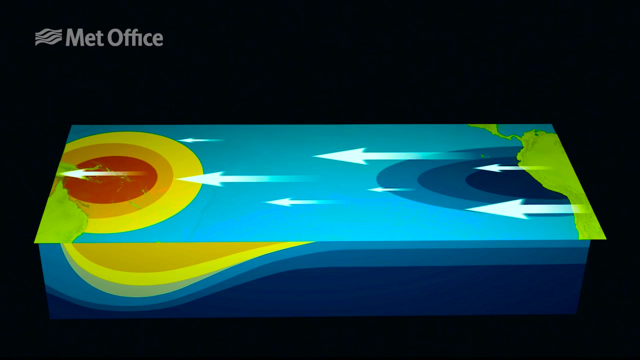 hemisphere, winter Neutral conditions occur in some years. During a La Niña year, ocean temperatures are lower than normal in the eastern tropical Pacific. La Niña develops when stronger-than-normal easterly trade winds push the warmest water further towards the western tropical Pacific and increase the upwelling of cold water near South and Central. 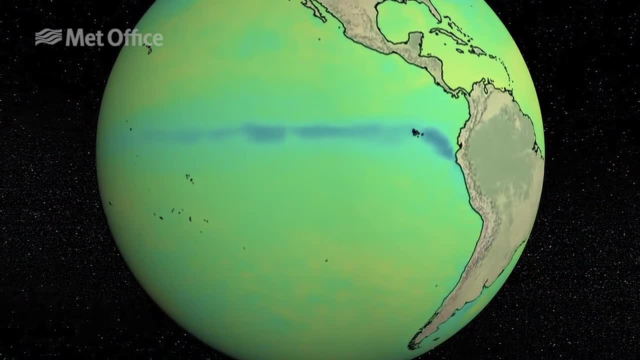 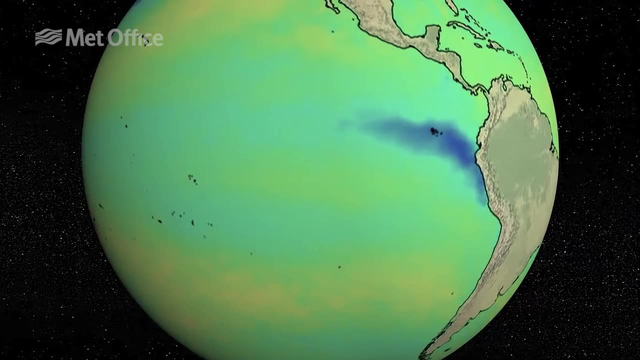 America in the east Sea surface temperatures in the east drop below normal. This cooler water extends out from the coastline. The temperature drops below normal as the coastal temperatures increase and the temperature drops below normal. The temperature drops below normal for most of South America towards the central part. 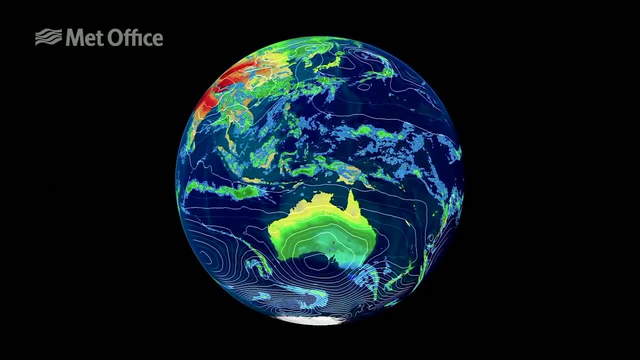 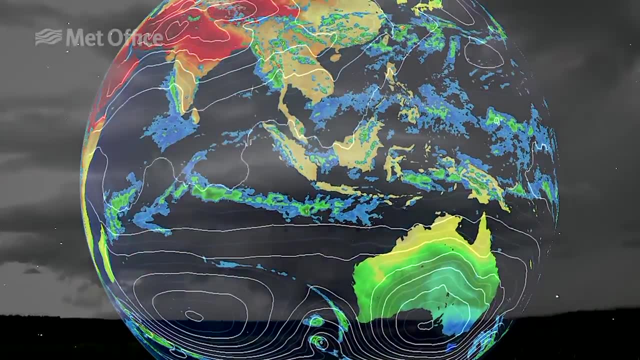 of the ocean. La Niña impacts global weather and tends to have opposite effects to El Niño. The impacts vary with season, but parts of Australia and Indonesia are typically wetter than normal during La Niña. Equatorial parts of South America are also often wetter than normal.